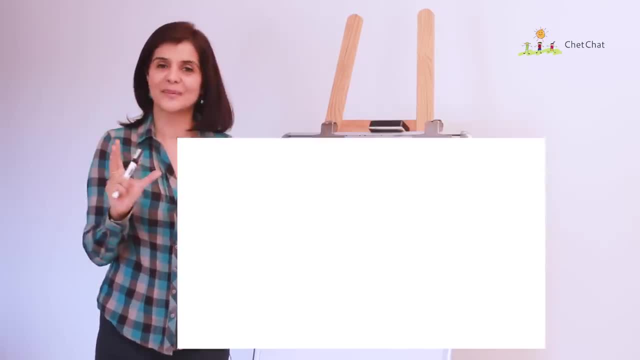 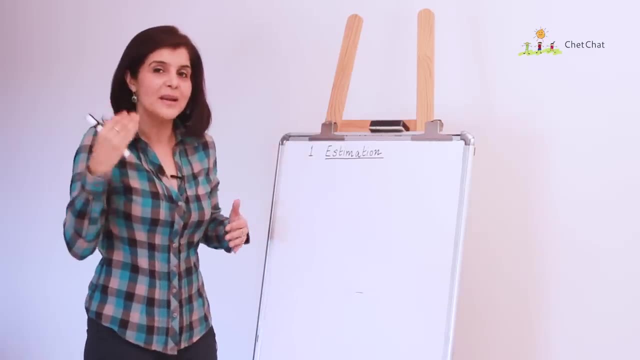 off. or we walk into a store and it announces 30% off And we're freaking out that. what does it exactly mean? Well, it's not an estimate, mentally right there in the store or the restaurant. So what is 4% of 250?? 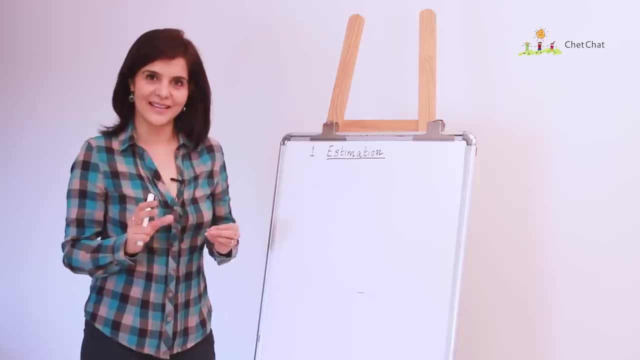 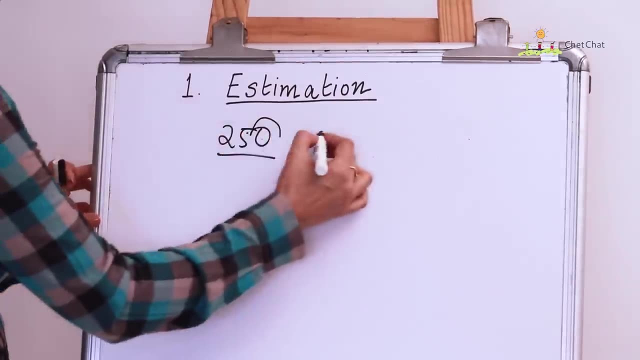 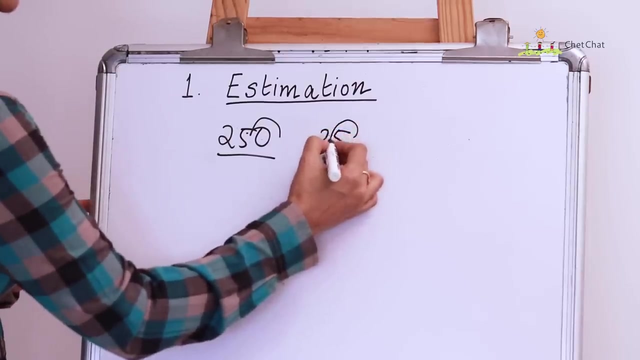 Now, before we jump into the answer, how about we try estimating that answer? Let's take 10% of 250, and 10% would mean 25,, right? We all know that? Now, what is 1% of 250?? That would mean 2.5.. And if we want 4%, then it's. 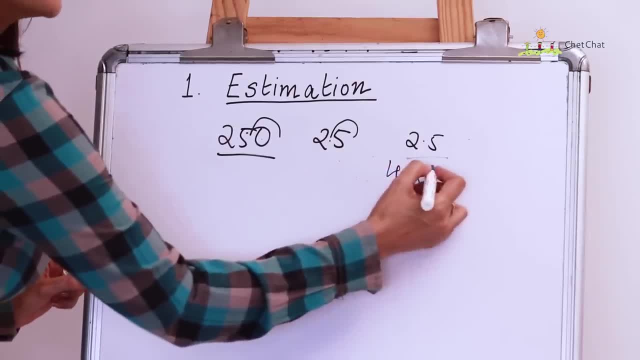 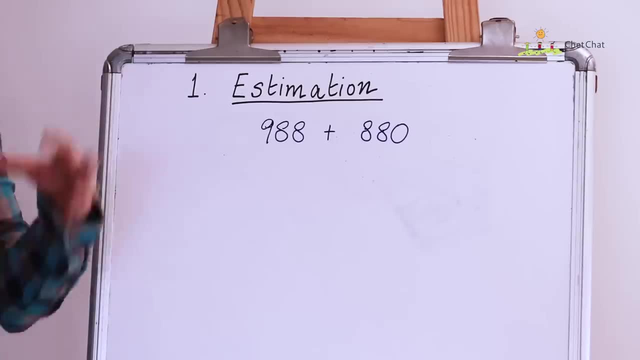 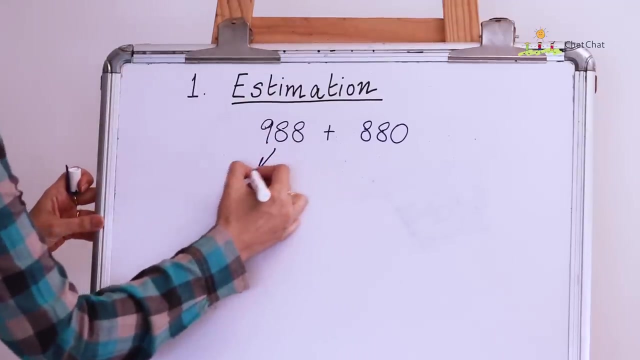 4 times of 1%, which is 4 times of 2.5,, which is 10.. Okay, let's try another exercise in estimation Now, before you start adding all these big numbers, let's try to take them to the nearest 100.. So I would take: 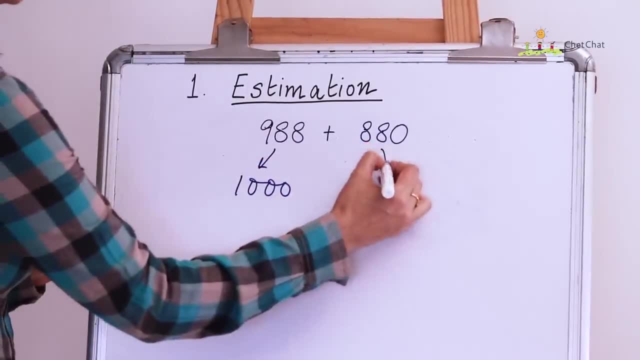 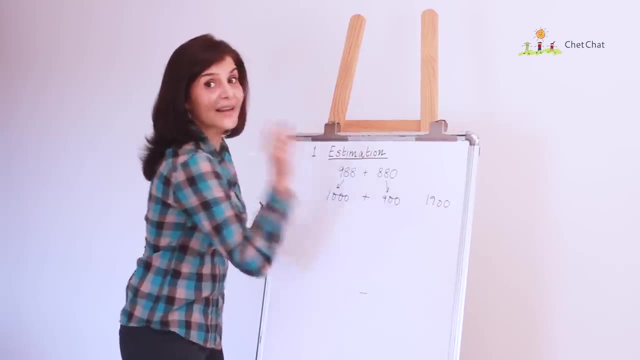 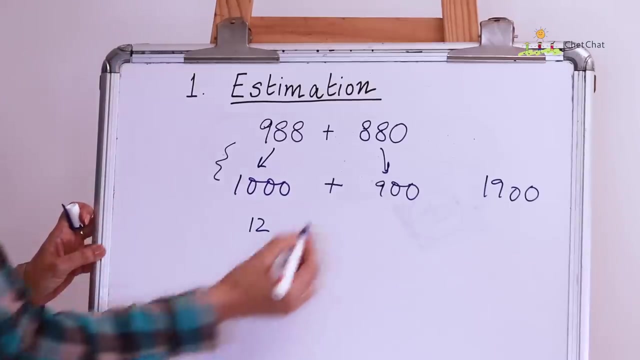 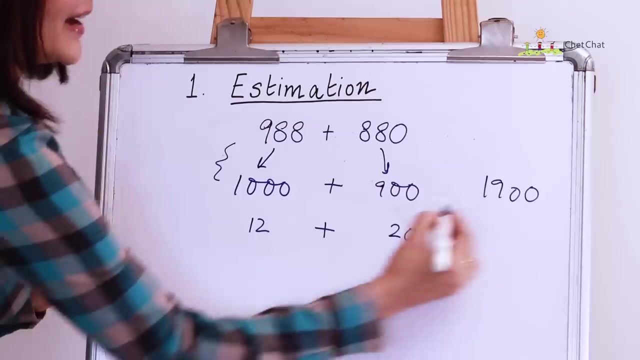 988 up to 1000 and I would take 880 up to 900 and I would add them up and I would get 1900.. Now, how much have I added Here in order to get a 1000, I've added 12 to 988 and I've added 20 to 880 to get 900.. So I need to subtract this. 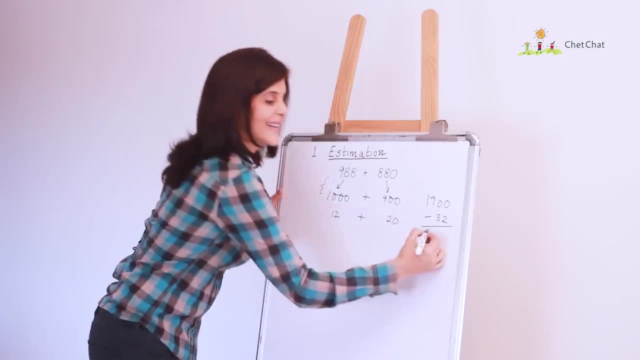 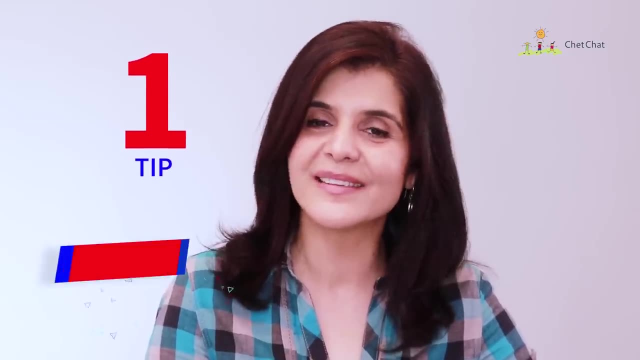 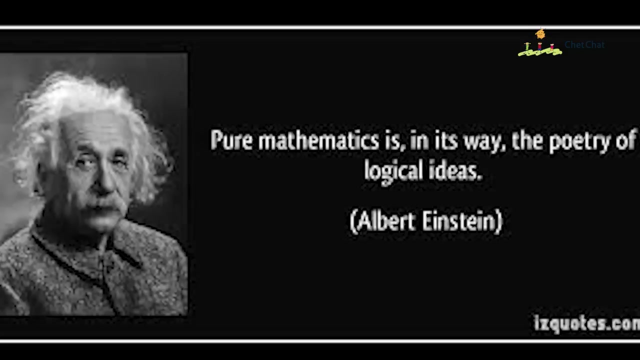 32 from 1900 and I get 1868.. Wasn't that easy. Tip number one: visualize, don't memorize. So Albert Einstein once said that pure math is actually like a poetry of logical reasoning. So don't look at math as. 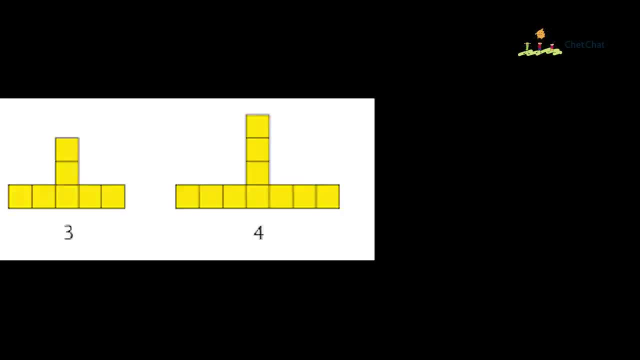 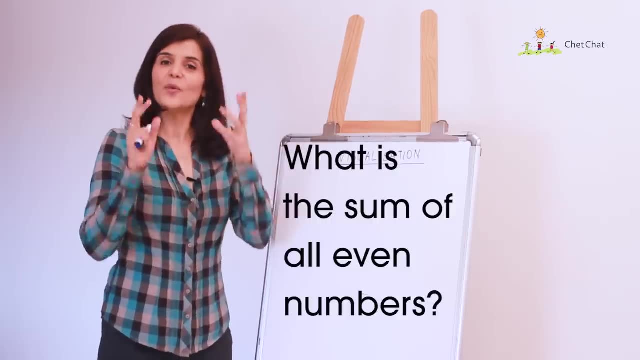 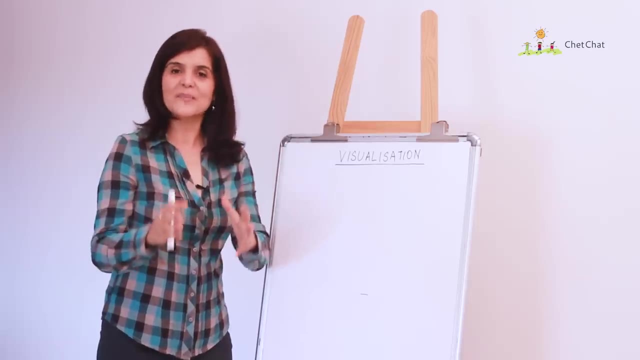 cramming up all those formulae. Instead, look at it like a storybook or a pattern, and that will help you enhance your logical reasoning. Okay, so what is the sum of all even numbers from 0 to 100?? Okay, let's break that down. What is the sum of? all even numbers from 0 to 10?? Now there are four even numbers between 0 and 10.. Which are 2,4,6 and 8.. Let's visualize these numbers. So reach to, let's draw two, And if I take four, it's-. 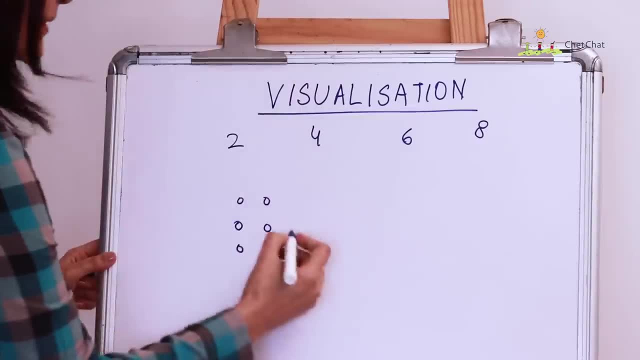 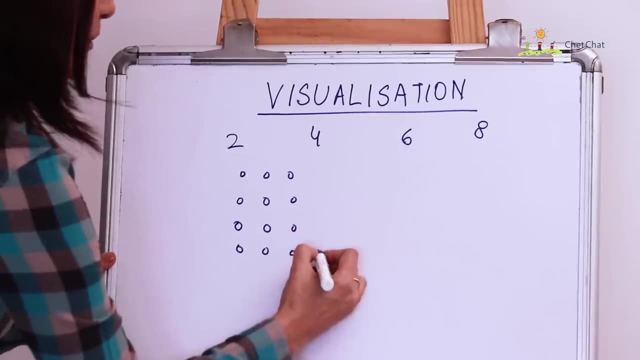 one, two, three, four, And If I take six, it's one, two, three, four, five, six, And if I take 8, it's one, two, three, four, five, 6,, 7,, 8.. 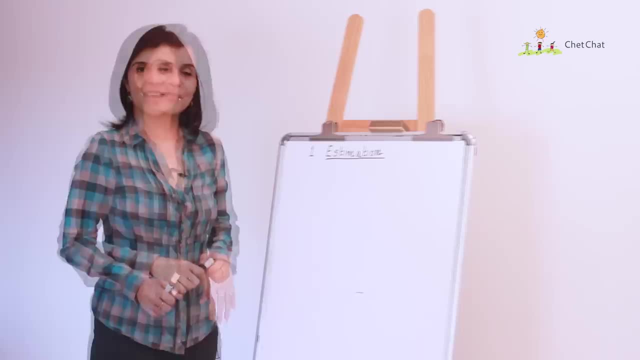 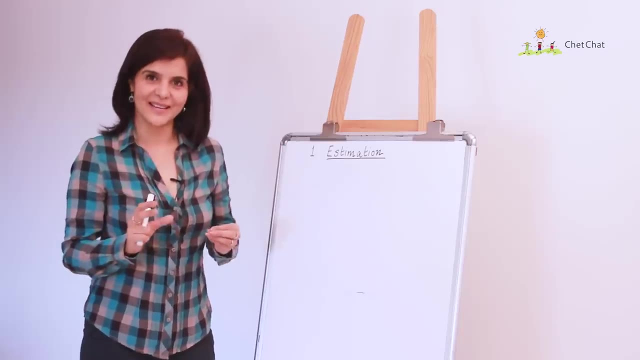 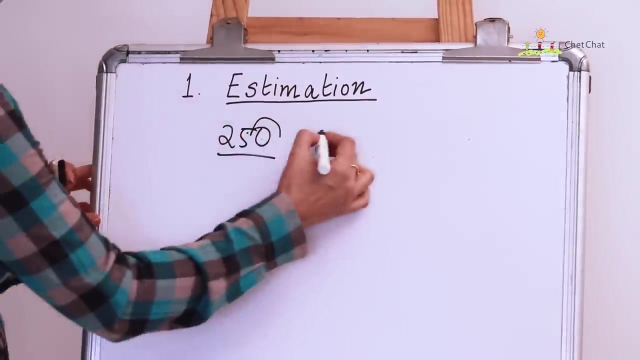 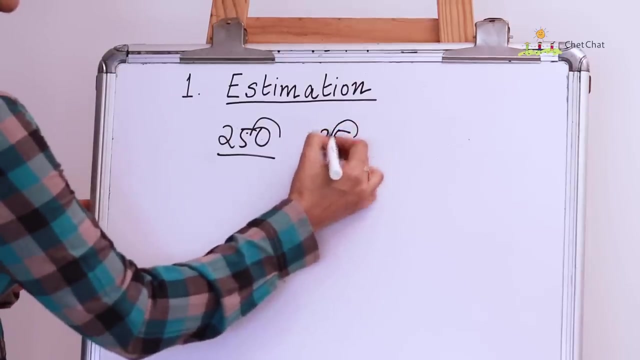 mentally right there in the store or the restaurant. So what is 4% of 250?? Now, before we jump into the answer, how about we try estimating that answer? Let's take 10% of 250, and 10% would mean 25,, right, We all know that. Now what is 1% of 250?? That would mean 2.5. And if we want 4%, then it's 4 times. 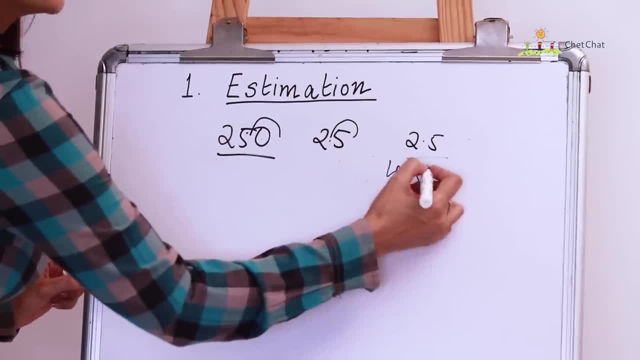 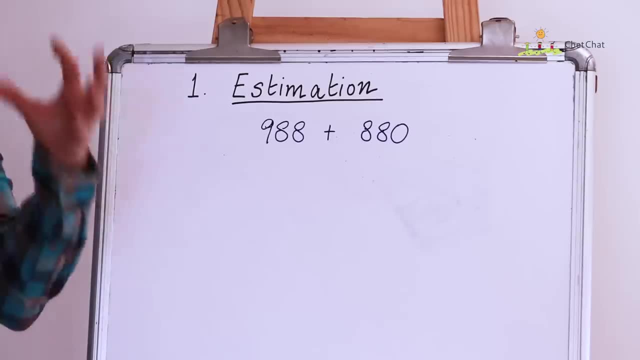 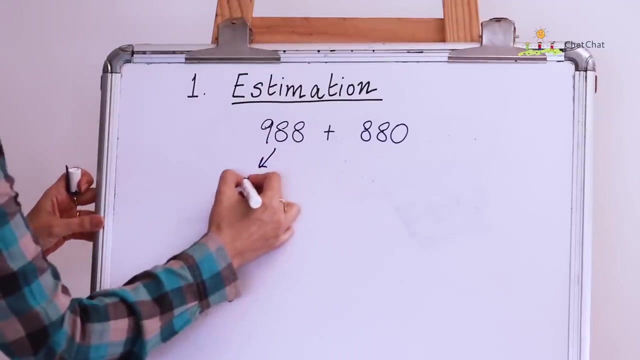 of 1%, which is 4 times of 2.5, which is 10. okay, let's try another exercise in estimation now, before you start adding all these big numbers, let's try to take them to the nearest hundred. so I would take 988 up to thousand and I would take 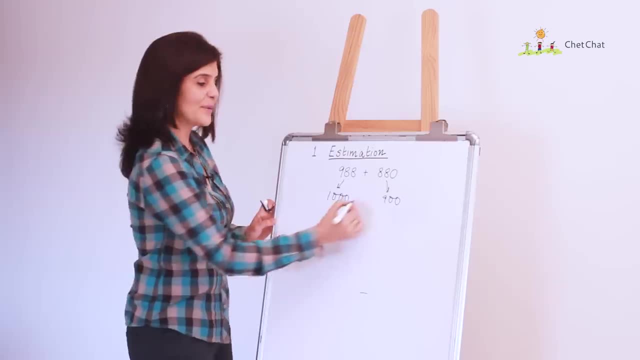 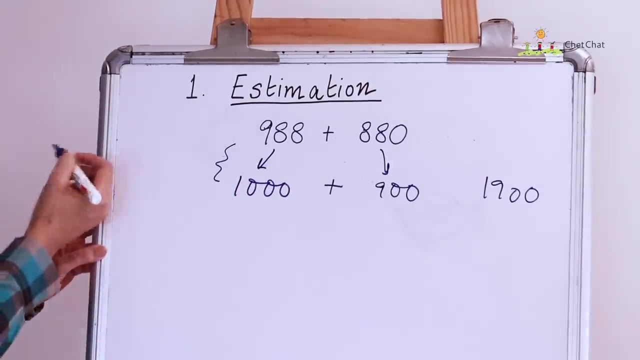 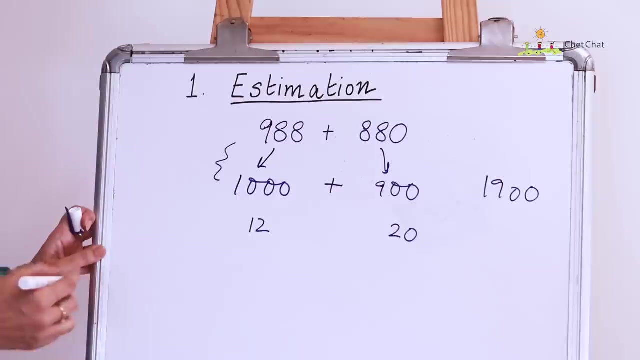 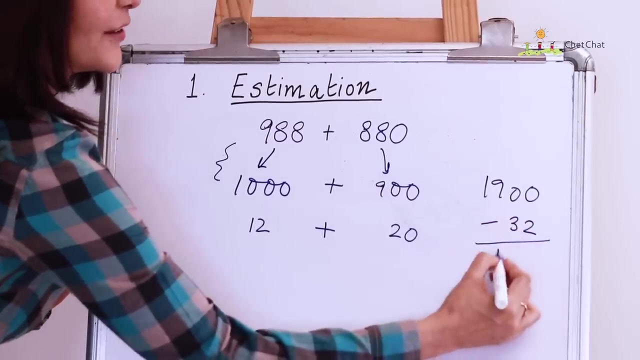 880 up to 900 and I would add them up and I would get 1900. now, how much have I added here in order to get a thousand? I've added 12 to 988 and I've added 20 to 880 to get 900. so I need to subtract this 32 from 1900 and I get 1868, wasn't? 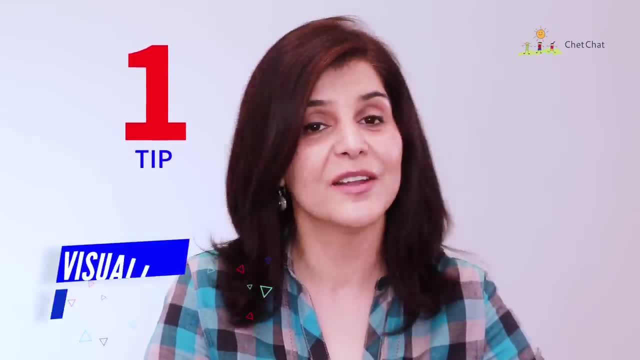 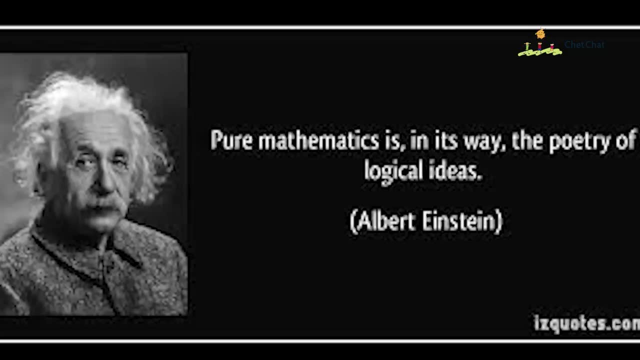 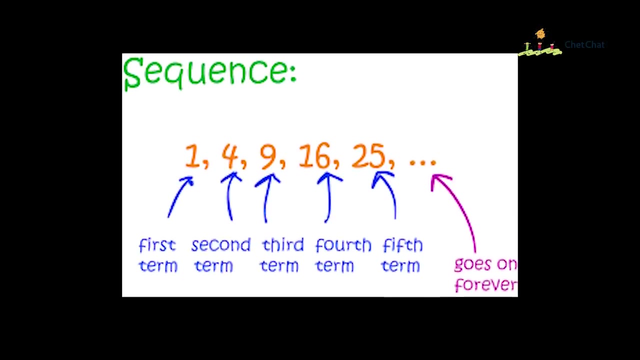 that easy tip number one: visualize, don't memorize. so Albert Einstein once said that pure memory is not a thing. pure math is actually like a poetry of logical reasoning. so don't look at math as cramming up all those formulae. instead, look at it like a storybook or a 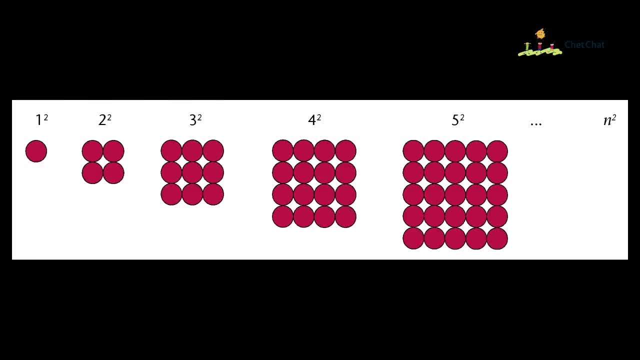 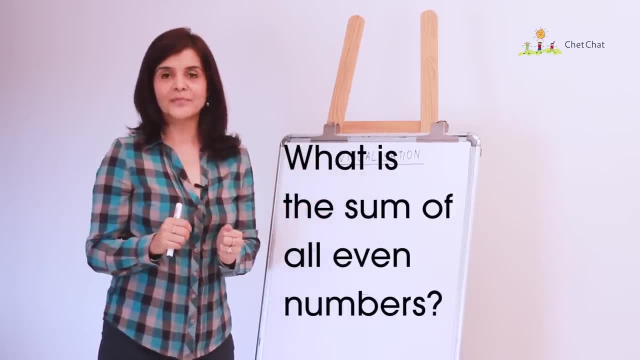 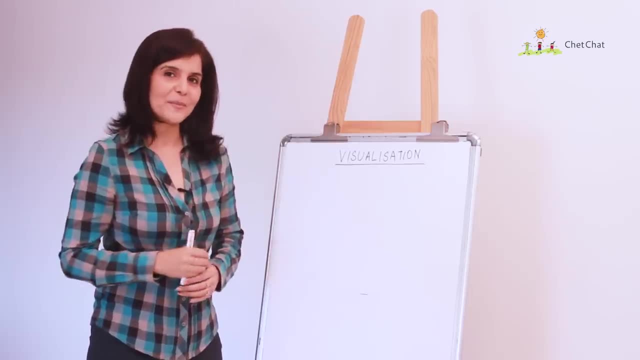 pattern and that will help you enhance your logical reasoning. okay, so what is the sum of all even numbers from 0 to 100, mm-hmm? okay, let's break that down. what is the sum of all even numbers from 0 to 10? now there are four even numbers. 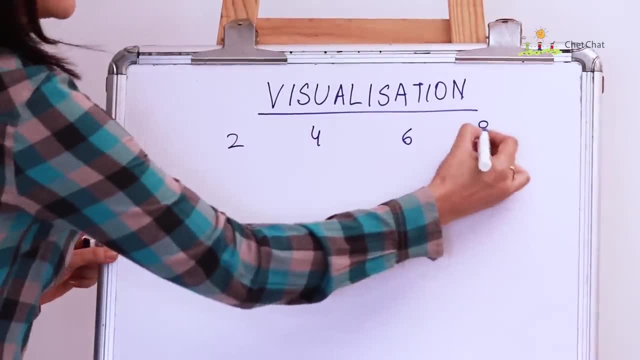 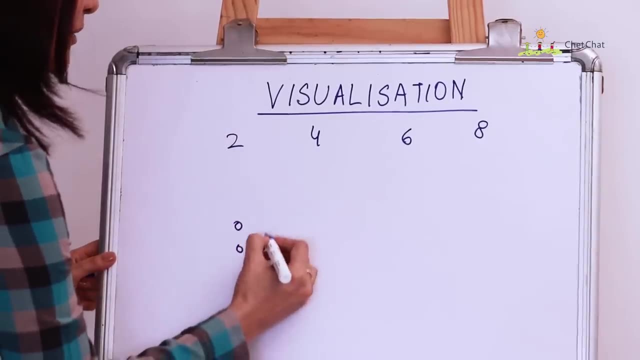 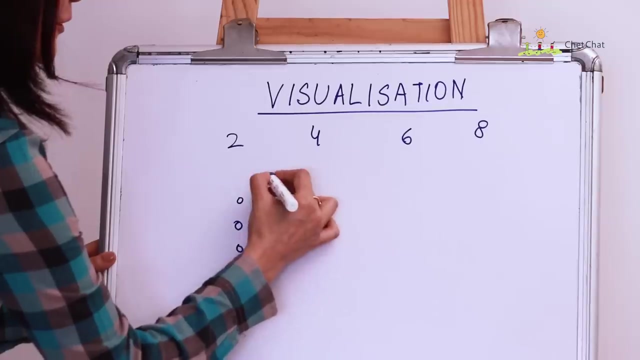 which are 2, 4, 6 and 8. let's visualize these numbers. so 2, let's draw 2, and if I take 4, it's 1, 2, 3, 4, and if I take 6, it's 1, 2, 3, 4, 5, 6, and if I take 8, it's 1, 2, 3, 4. 5, 6, 7, 8. so what have I got? here is a sum of all even numbers from 0 to 900, and I get a square of 4 into 5, which is 20, and now you can begin to guess the formula. 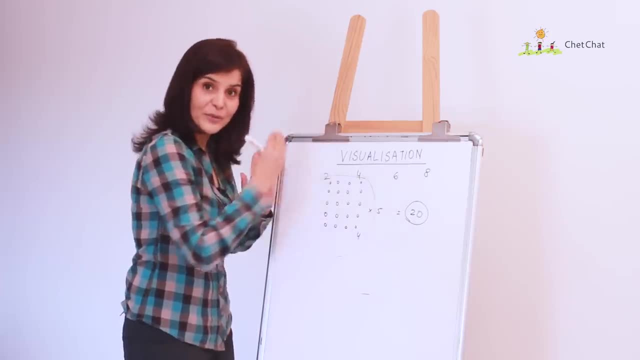 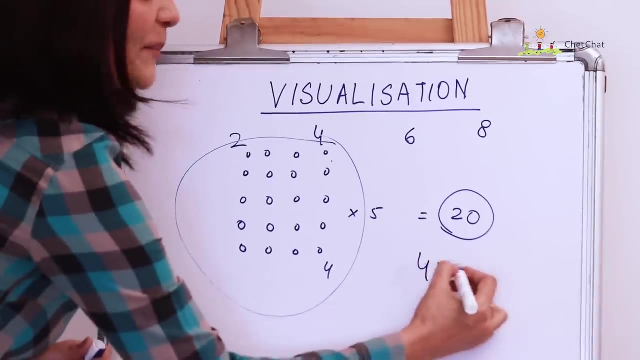 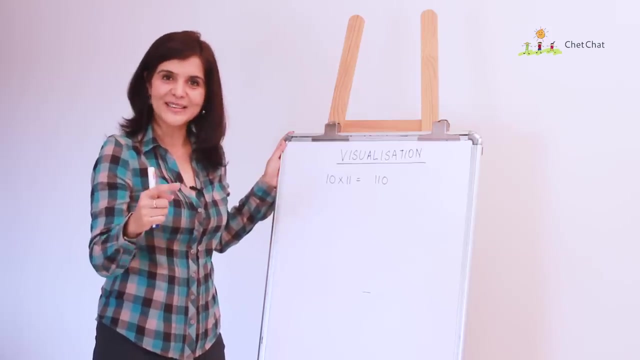 it's the number of even numbers between 0 and 10. so in this case it's 4 even numbers between 0 and 10 multiplied by n plus 1, that is 5, which is equal to 20. now try it with all numbers. it's not exactly this formula. 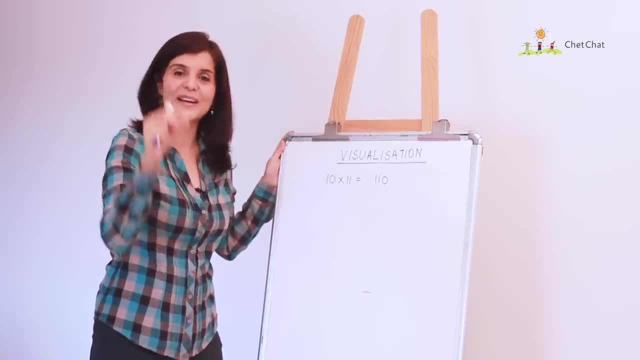 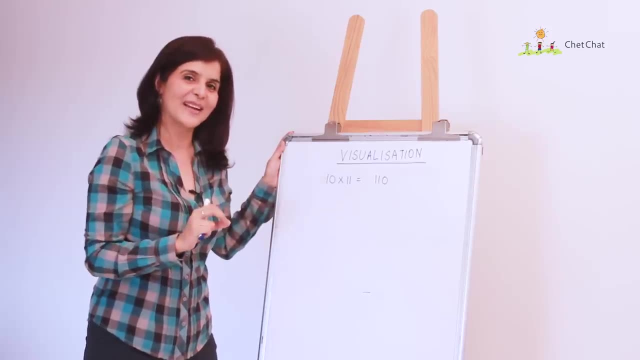 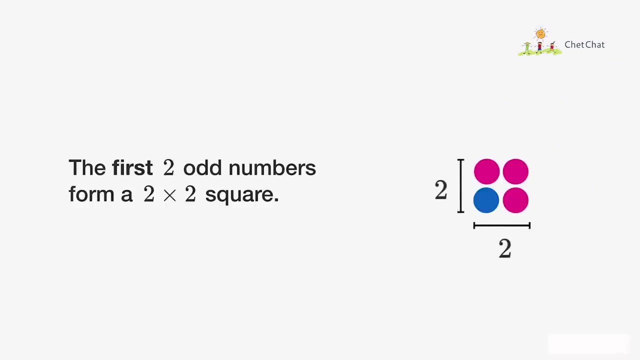 it's something different and I want you to put that formula in the comment section below: what is the sum of the odd numbers between 0 and 10 and what did you get as the formula? and before we get to the balance, three tricks: don't forget to tell me which of 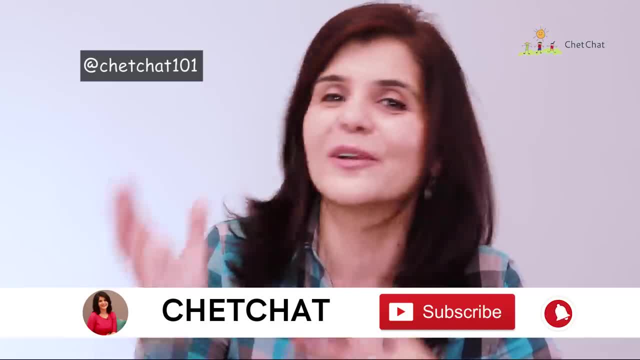 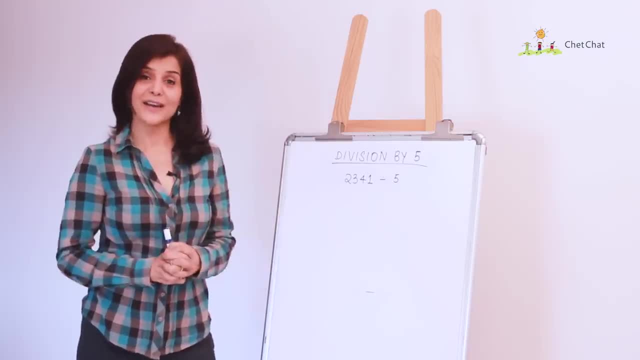 the six was your favorite, or if there's any other trick that you love, put everything down for me in the comment section below this video. trick number three: division by 5. what is 25 by 5? 5, that's easy. but what is 2, 3, 4? 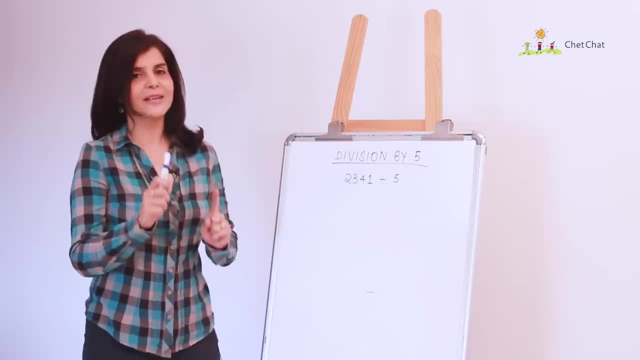 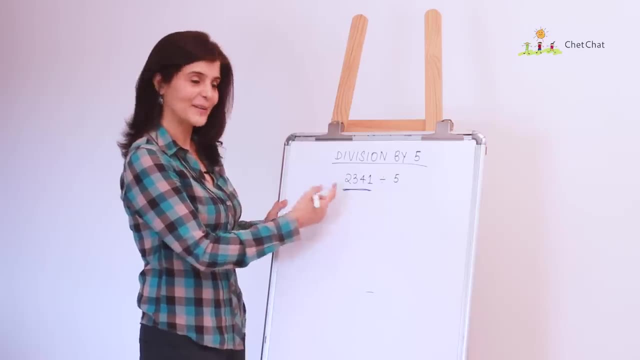 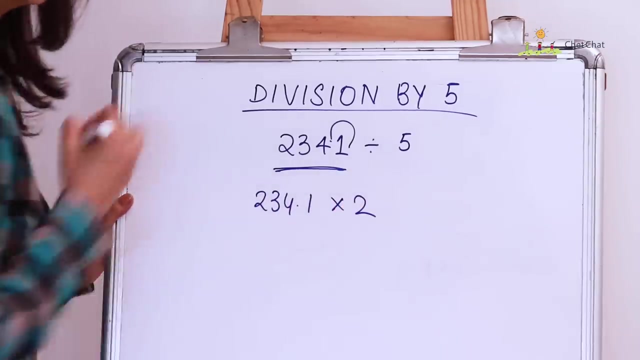 1 by 5. hmm, okay, let's remember, 5 is 10 by 2, so how about we first divide this by 10? so 2, 3, 4, 1 divided by 10 is 2, 4.1, and now I can multiply this by 2 and I've got 468.2.. Wasn't that quick, Okay, and now's your 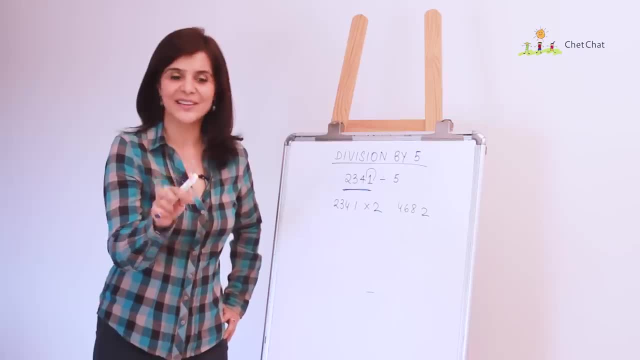 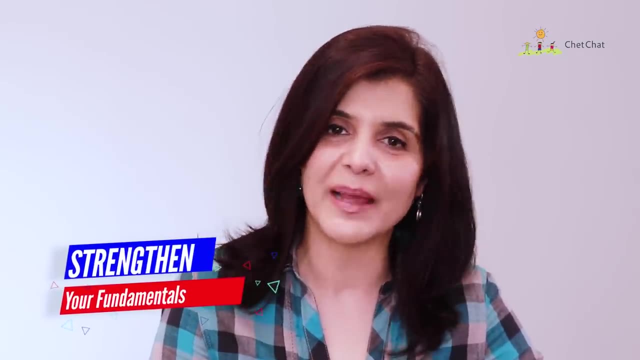 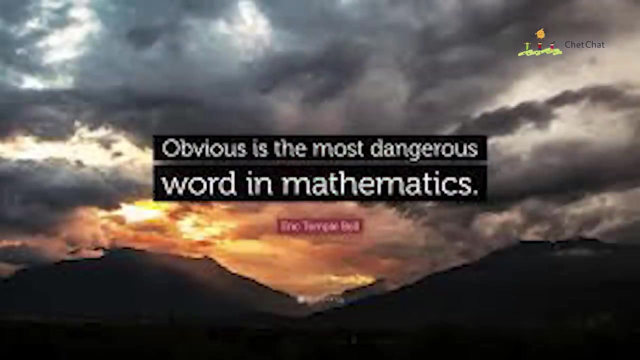 turn 897 by 5, the fastest calculation in the comments box right now. Tip number two: strengthen your fundamentals. Eric Temple Bell, a famous Scottish mathematician, once said that obvious is the most dangerous word in mathematics. So go back to basics, strengthen your fundamentals. 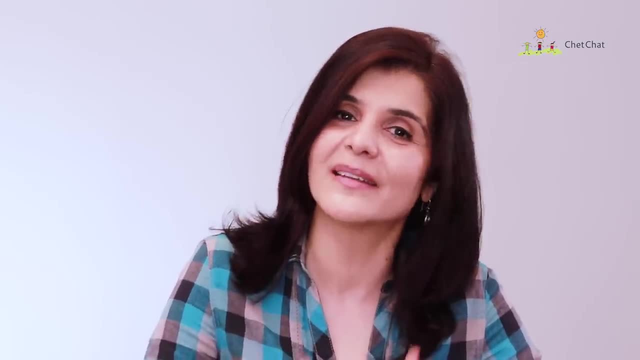 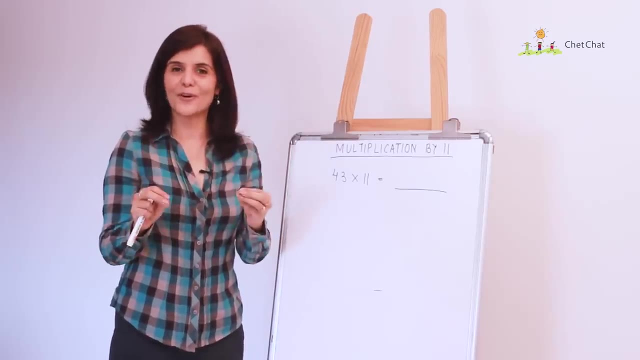 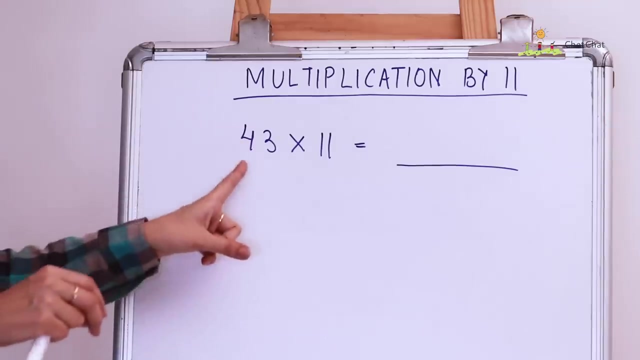 and practice, practice, practice to become this expert, slowly and gradually. Okay, now a very simple trick. Trick number four is multiplication by 11, and I'm going to take a very basic example right now to explain this. Let's take 43 into 11, and when we multiply it, the units place. 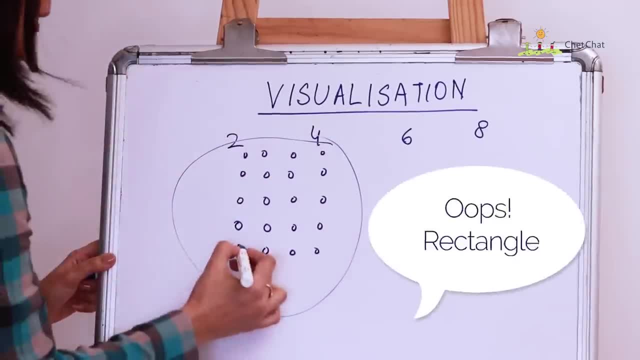 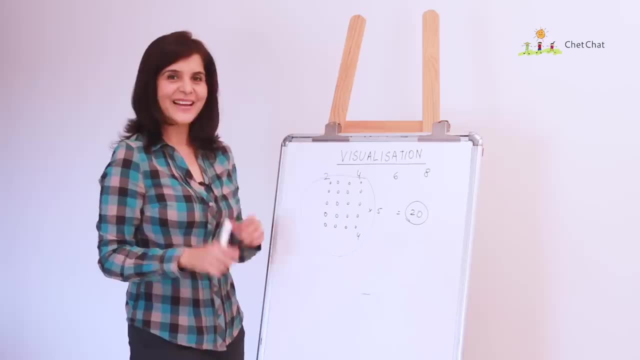 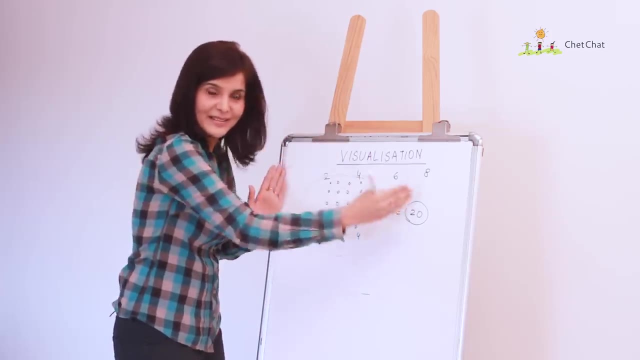 Therefore, what- I ve gotten here is a square of 4 into 5, which is 20, and now you can begin to guess the formula: it's the number of even numbers between 0 and 10. so in this case, it's 4 even numbers. 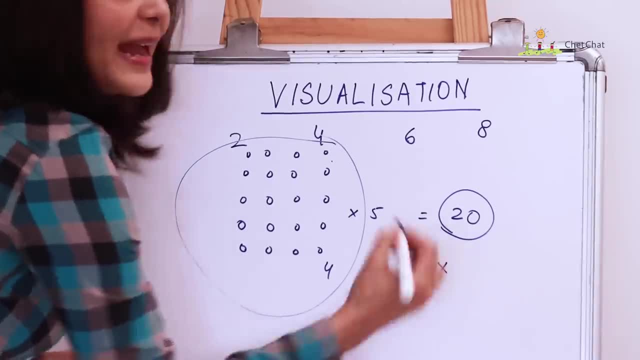 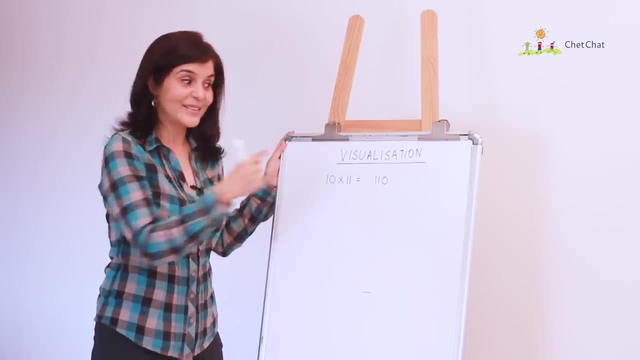 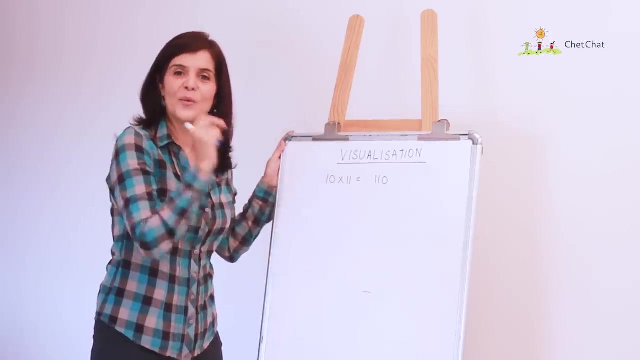 between 0 and 10. multiplied by n plus 1, that is 5, which is equal to 20. now try it with odd numbers. it's not exactly this formula. it's something different and I want you to put that formula in the comment section below: what is the? sum of the odd numbers between 0 and 10. and what did you get as the formula? and before we get to the balance table, three tricks. don't forget to tell me which of these tricks was your favorite, or if there's any other trick that you love. put everything down for me in the 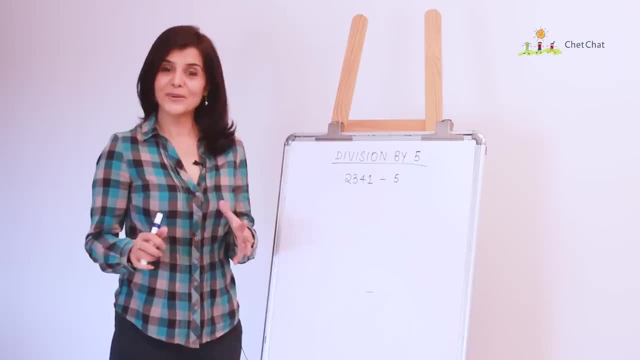 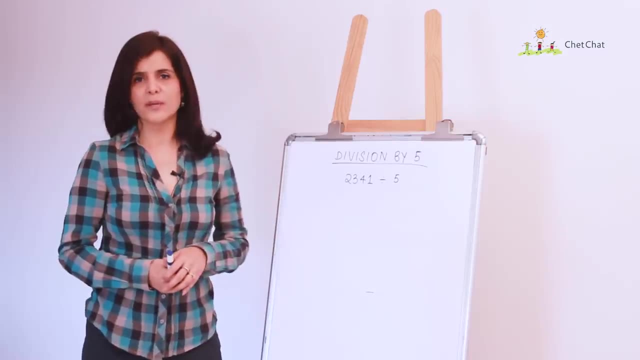 comment section below this video trick. number three: division by 5. what is 25 by 5? 5, that's easy. but what is 2, 3, 4, 1 by 5? hmm, okay, let's remember, 5 is 10 by 2. so 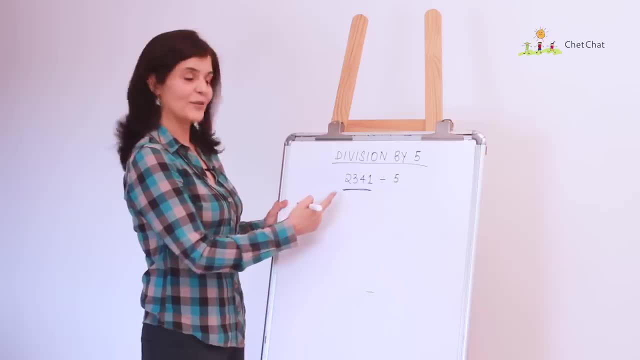 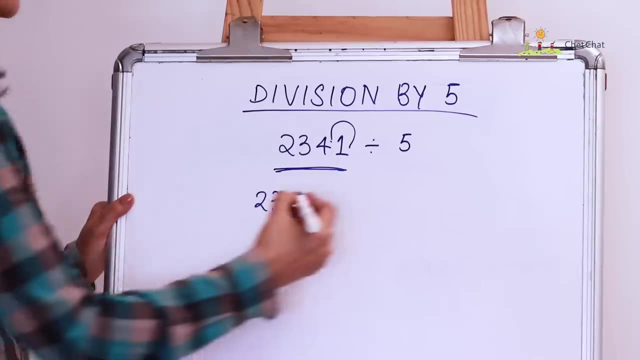 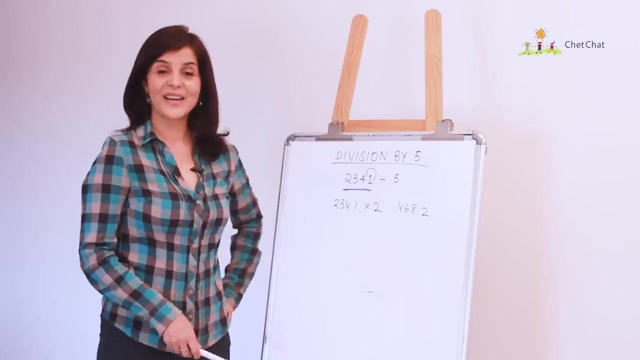 how about we first divide this by 10? so 2, 3, 4, 1 divided by 10 is 234 point 1. and now I can multiply this by 2 and I've got 468 point 2. wasn't that quick, okay. and now is your turn: 897 by 5, the fastest calculation in. 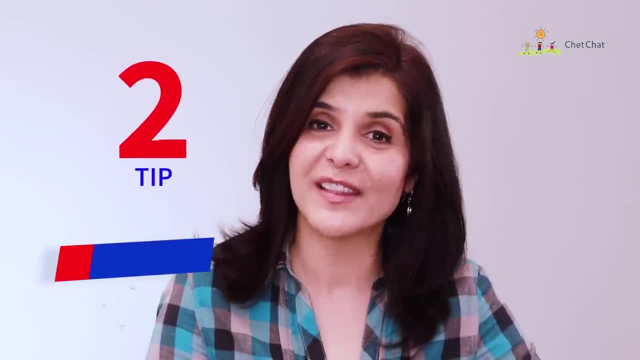 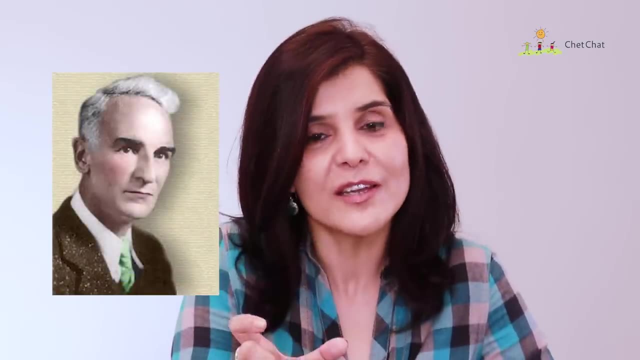 the comments box right now. tip number 2: strengthen your fundamentals. Eric Temple Bell, a famous Scottish mathematician, once said that obvious is the most dangerous word in the world. Tip number 2: strengthen your fundamentals. Eric Temple Bell, a famous Scottish mathematician, once said that obvious is the most dangerous word in the world. 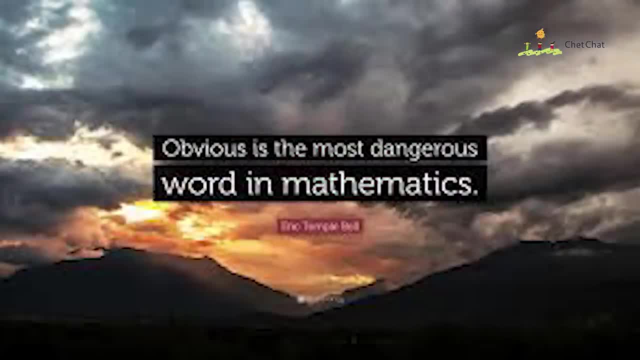 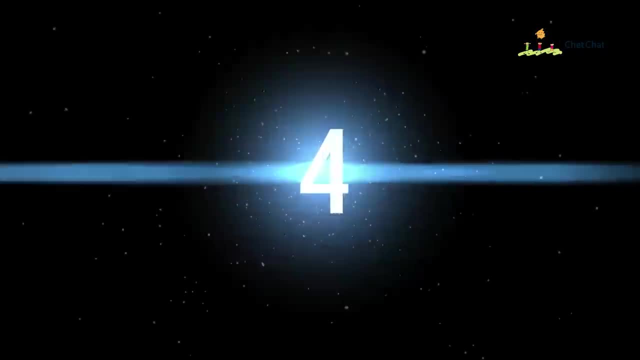 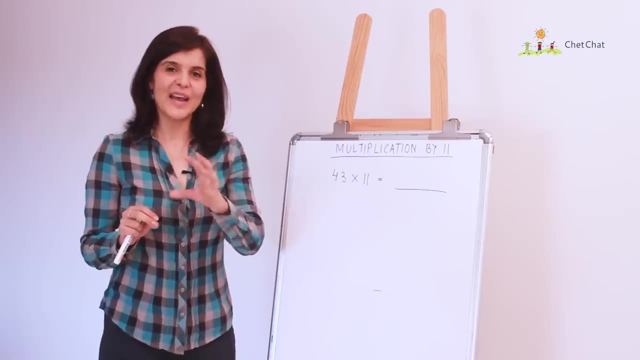 in mathematics. so go back to basics, strengthen your fundamentals and practice, practice, practice to become this expert, slowly and gradually. okay now a very simple trick. trick number four is multiplication by 11, and I'm going to take a very basic example right now to explain this. let's take 43 into. 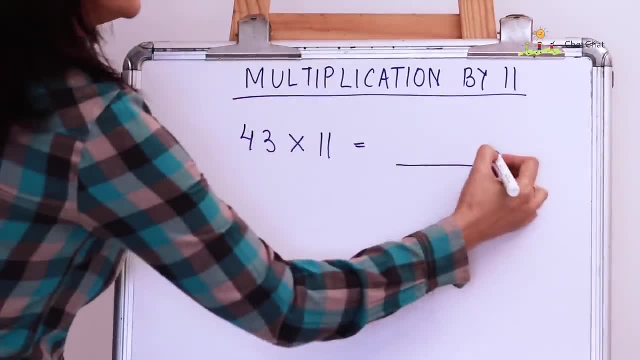 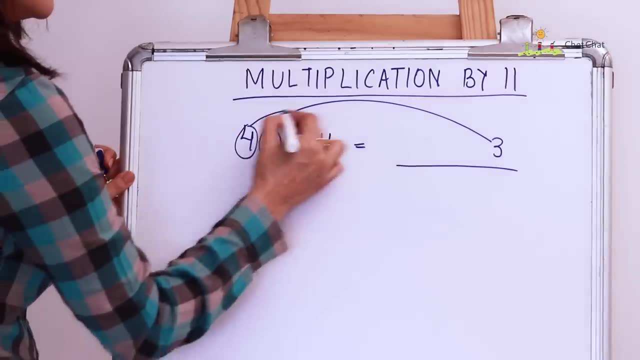 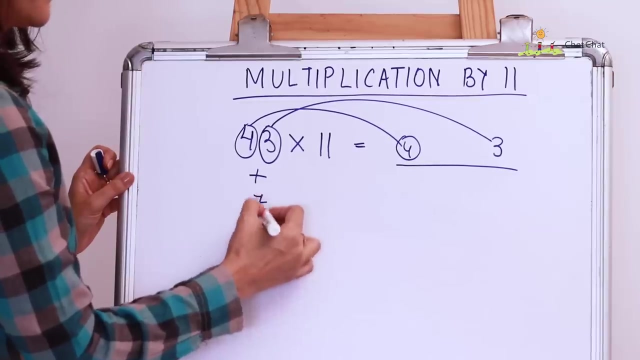 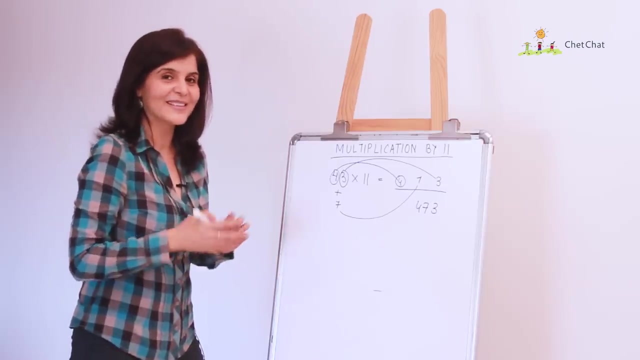 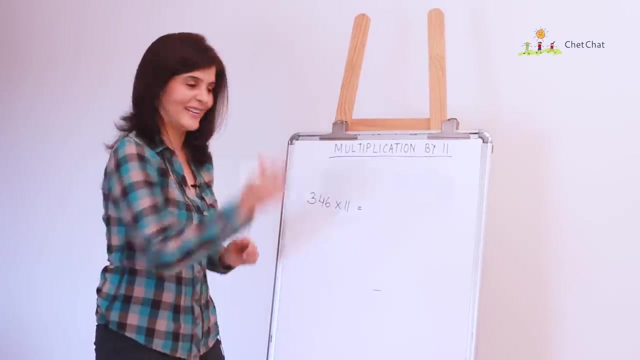 11, and when we multiply it, the units place is this: the first digit is this and the digit in the middle is the sum of these two: 473. now that sounds too easy, so let's take a little complicated example to see if that really works. okay, we've got a bigger number here, 346 by 11. let's see. 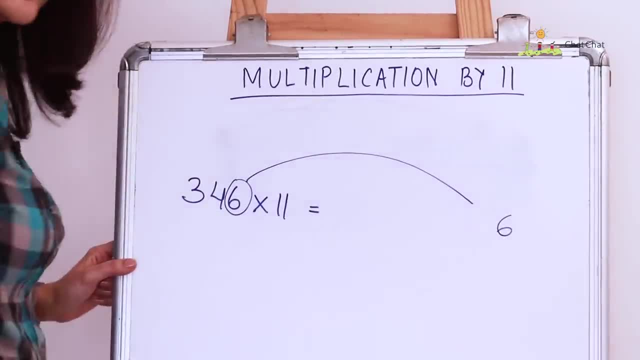 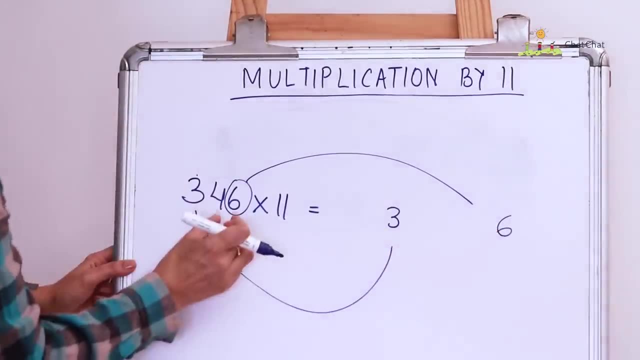 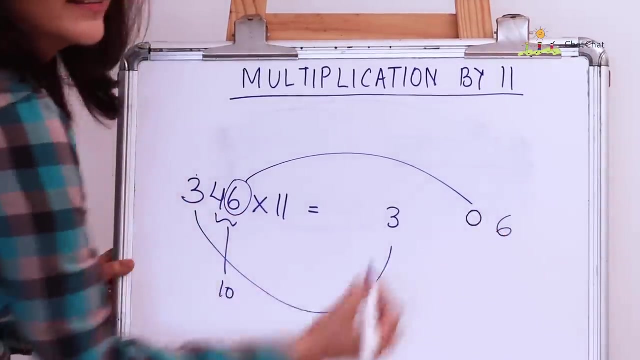 how it goes. so the units place is 6. the first digit is 3. now the number here is the sum of these two digits, which is 10. so I put 0 here and I keep the 1 for carry forward, and the number here is the. 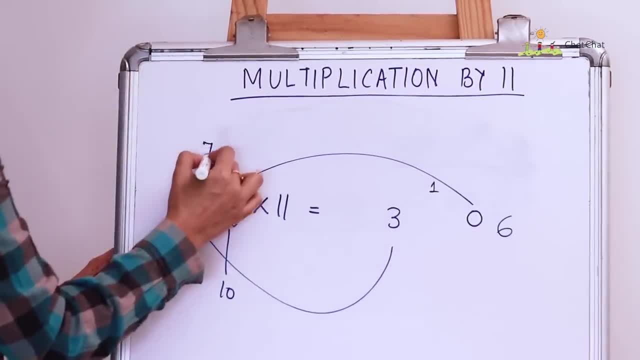 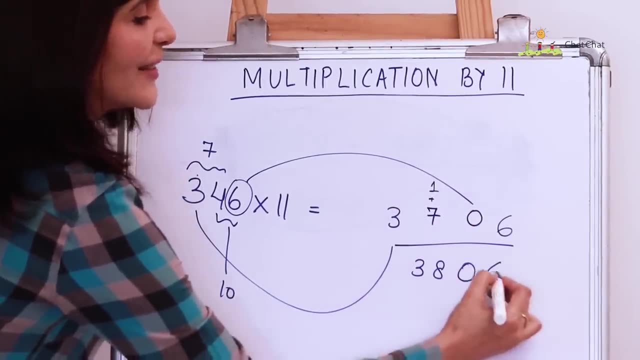 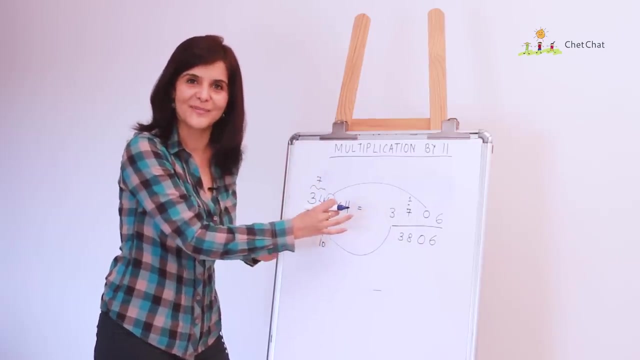 sum of these two digits, which is 7, and so the answer is 3 8 0, 6. this formula works, fail-proof. you just need to be careful about doing the carry forward every time. now, before we move on to the next tip, I wanted to remind you. 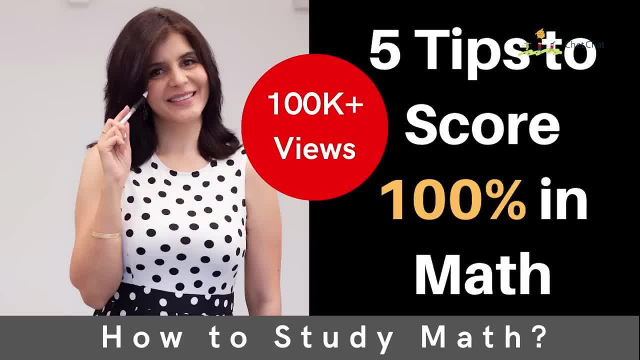 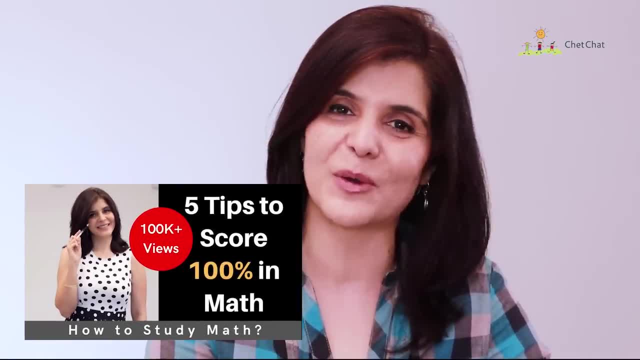 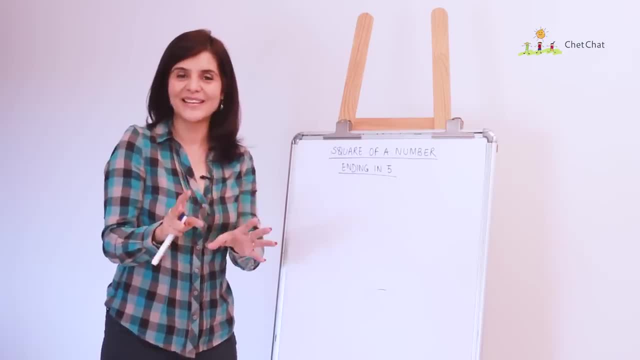 that we have a video called the five tips to score a hundred percent in math and I'm dropping a link for you in the description box so you can go check that out once you finish watching this video. and trick number five is to find the square of any number ending in five. this magical trick will help you to score a hundred percent in math. 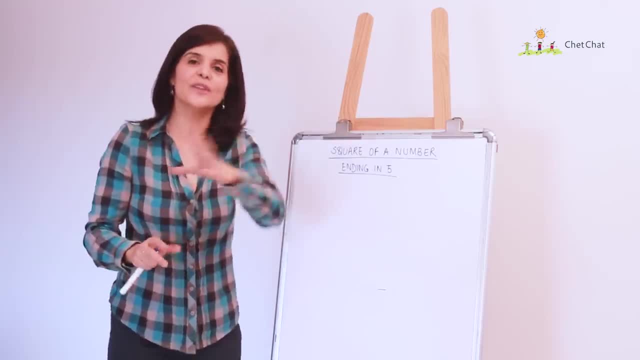 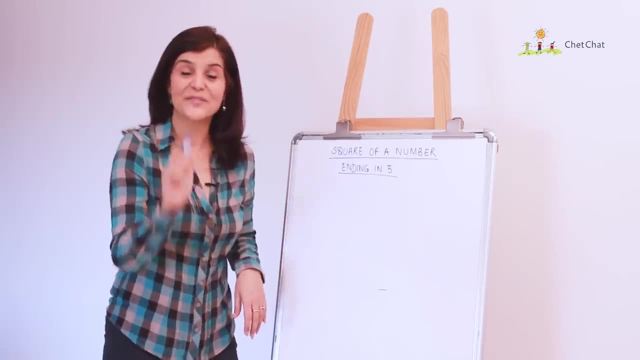 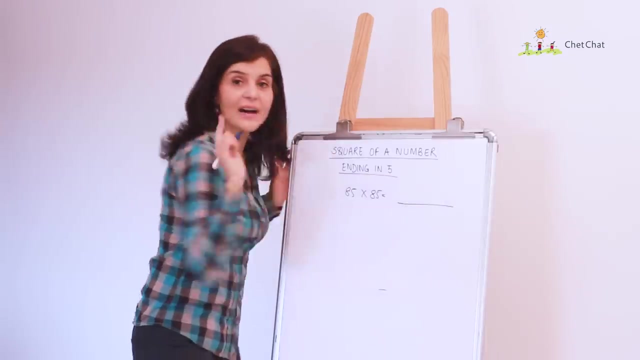 help you find the square at lightning speed. so what is the square of 85? quick write it down in the comment section right now. did you get 7 to 25? if you didn't, here's how we got it. so 85 into 85. now the last two digits will always. 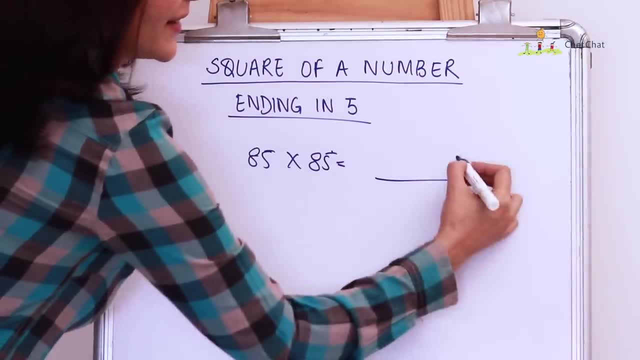 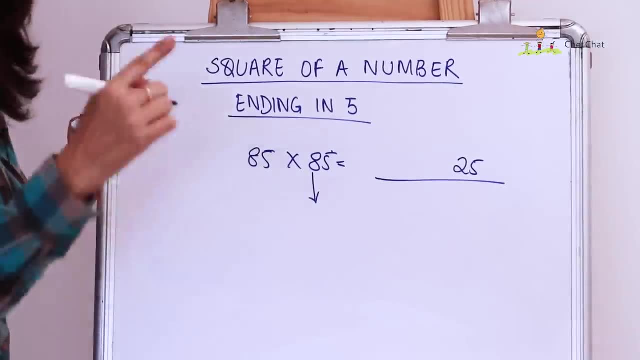 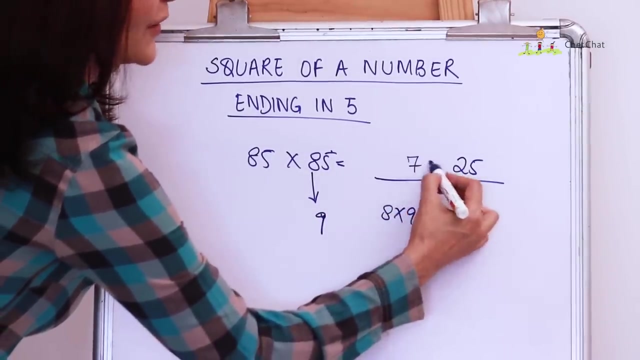 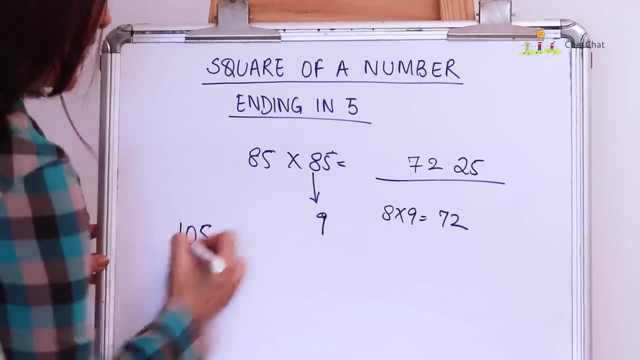 be 25. the square of 5 is 25 and the first two digits will be 8 into the number that comes out of the square of 8.. after 8, which is 9, so 8 into 9 is 72, and you've got 7, 2, 2, 5. let's try this with 105, so 105 a square. 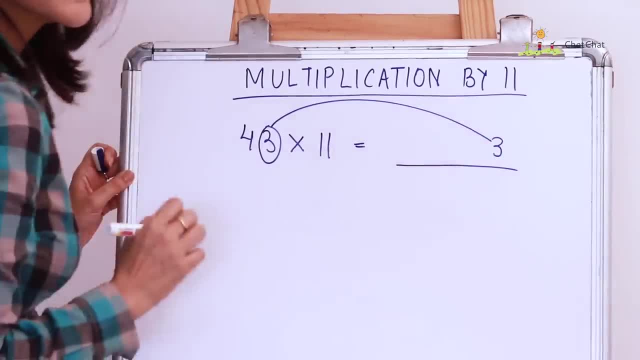 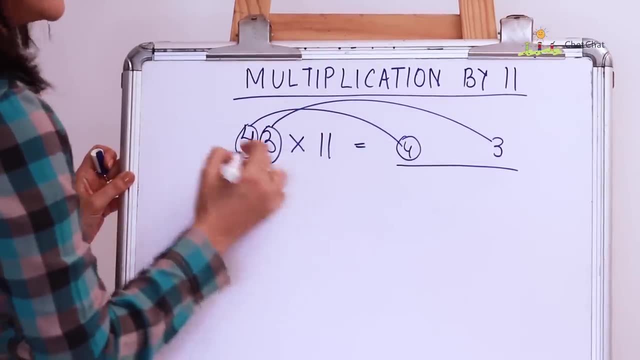 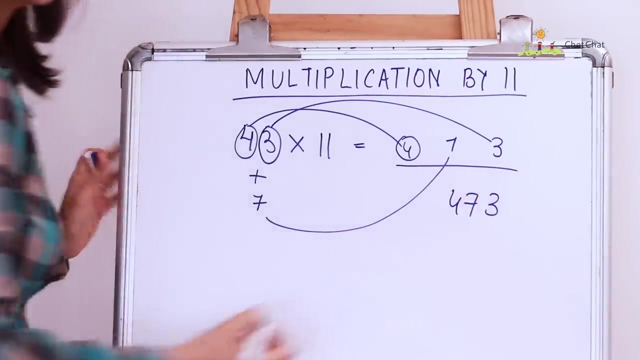 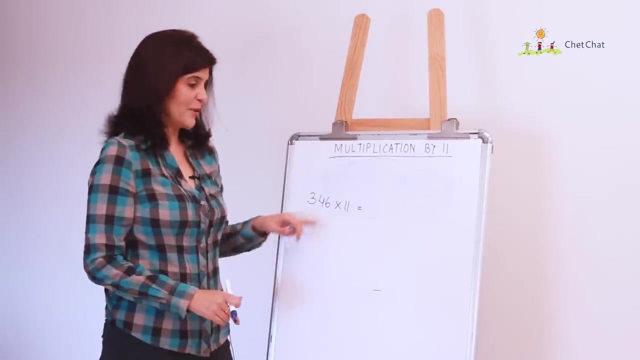 is this. The first digit is this, and the digit in the middle is the sum of these two: 473.. Now, that sounds too easy, So let's take a little complicated example to see if that really works. Okay, we've got a bigger number here, 346 by 11.. Let's see how it goes. So the units place: 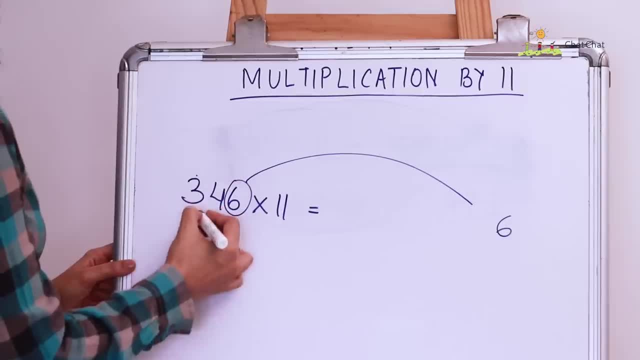 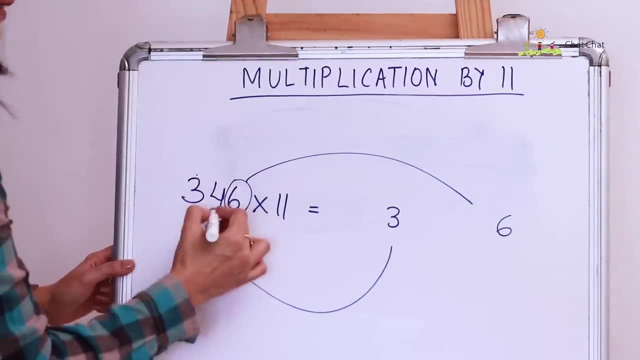 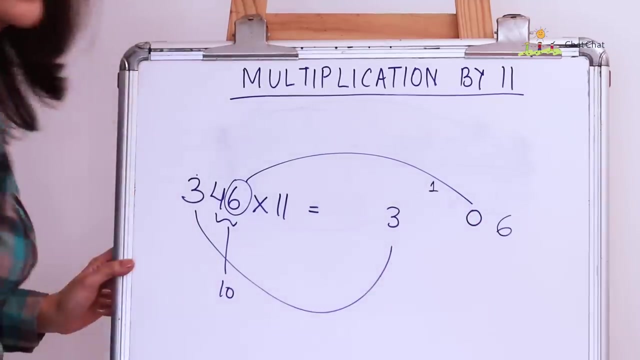 is 6,. the first digit is 3.. Now the number here is the sum of these two digits, which is 10.. So I put a 0 here and I keep the 1 for carry forward, and the number here is the. 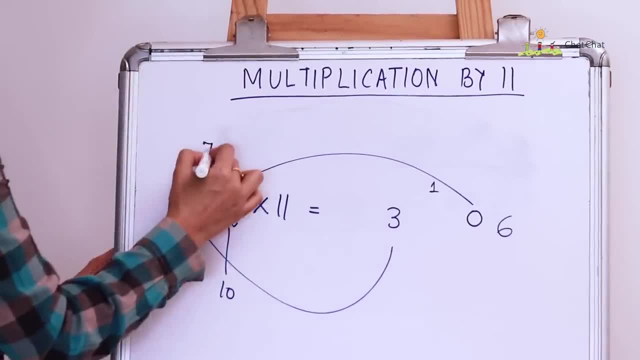 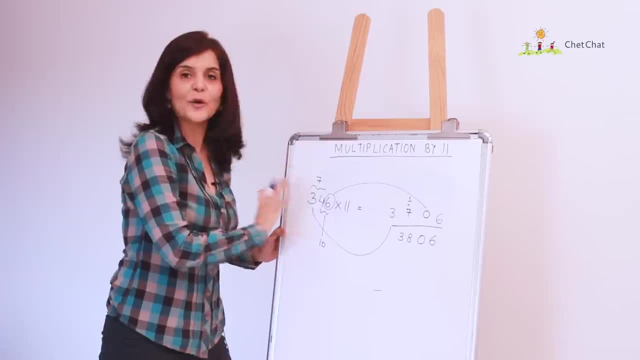 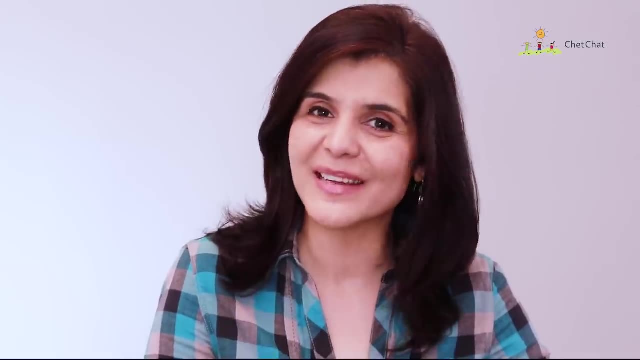 387.. Okay, so the answer is 387.. This formula works. fail proof. You just need to be careful about doing the carry forward every time. Now, before we move on to the next tip, I wanted to remind you that we have a video called The 5 Tips to Score 100% in. 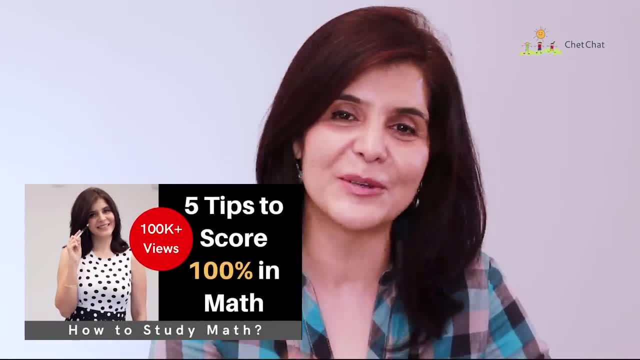 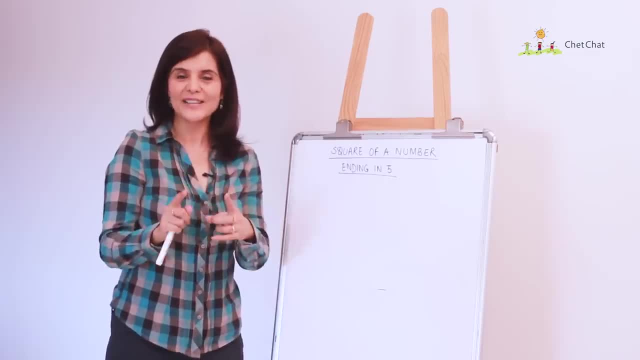 Maths- and I'm dropping a link for you in the description box so you can go check that out once you've finished watching this video. And trick No 5 is to find the square of any number ending in a number. So what we does is we does that by formula 1 times. 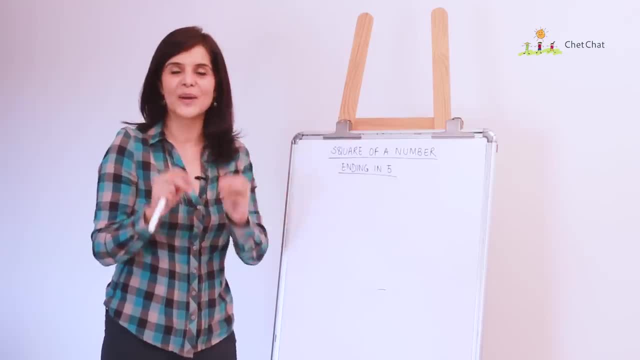 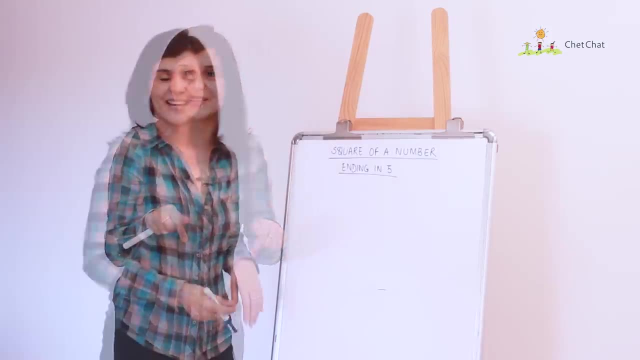 in 5.. This magical trick will help you find this square at lightning speed. So what is the square of 85?? Quick write it down in the comment section right now. Did you get 7, 2,, 2, 5?? If you didn't, 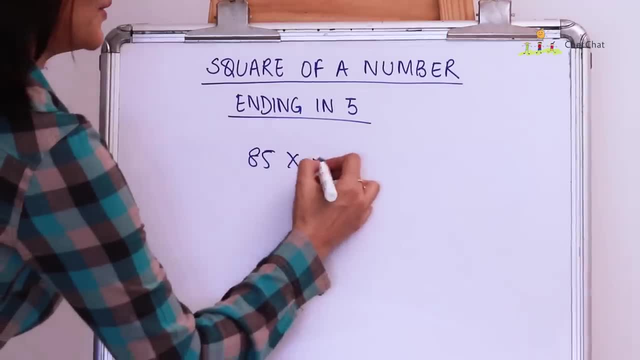 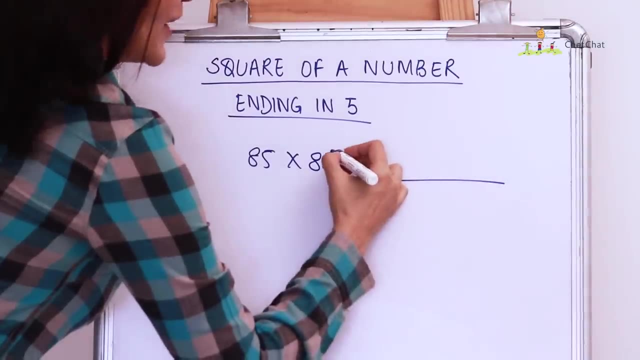 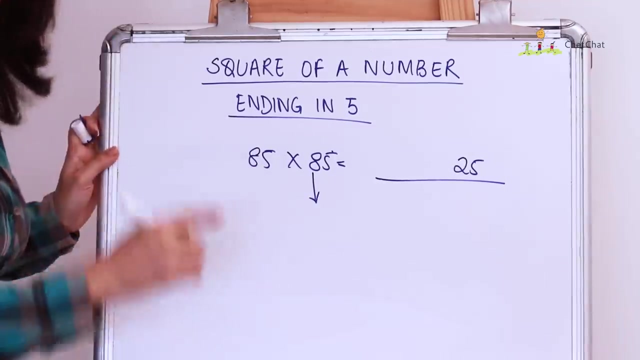 here's how we got it, So 85 into 85.. Now the last two digits will always be 25.. The square of 5 is 25, and the first two digits will be 8 into the number that comes after 8, which is 9.. So 8 into 9.